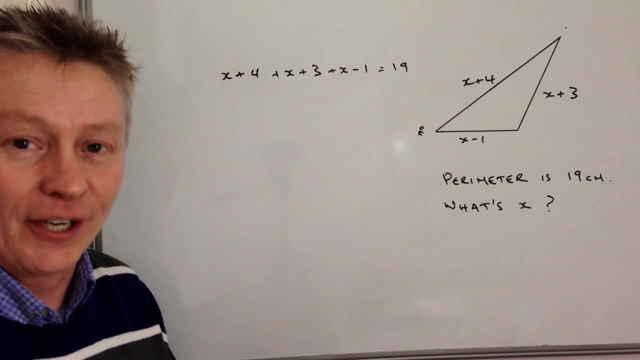 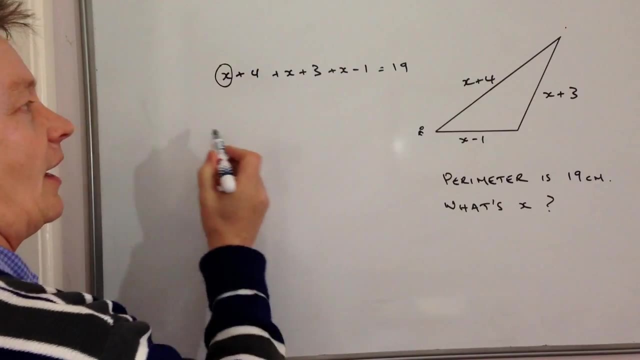 it's just a case of what they call gathering lines. OK, so you see this: down here we've got 8 x's drawn in the middle. That's because 0 and 10 with x, So it's busy. Let's say, I have x squared here and I've got x squared. 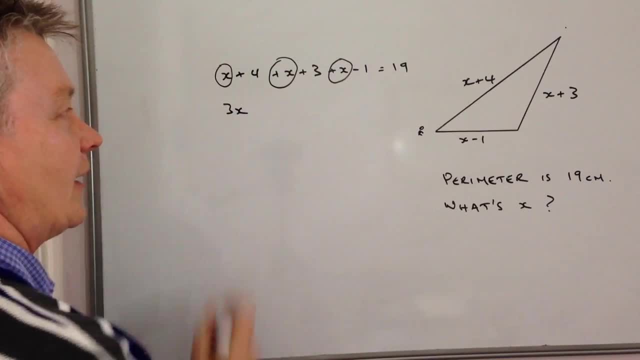 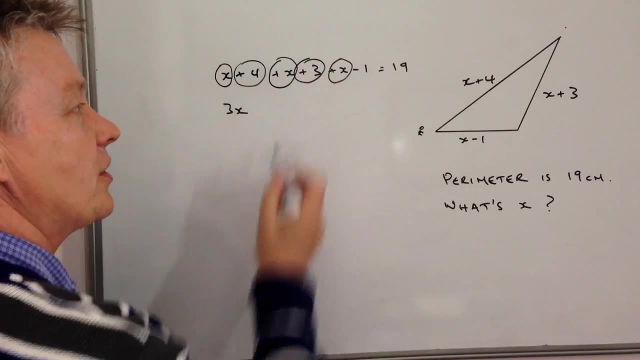 in the middle. So now I can just add x and 1,, 2,, 3,, 4,, 7,, 8,, 9,, 10 and 10 over 15,, 15,, 14 and 11. Together they make 16.. So if I add all of those xs together we end up with three xs, And then we look at the numbers themselves. So we've got plus 4, plus 3, which is 7, and minus 1, which is going to be 6. E年的, and then I will need 12 times 3, which is minus. 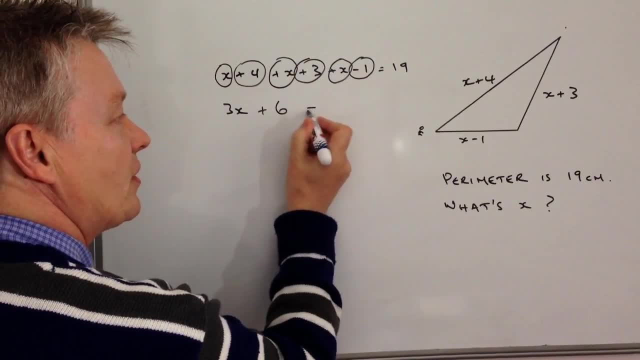 7.. So then I will need all the numbers written down, Let's say something like 23, and then then I spinning a circle with times From every sum, and if I do a diagonal I will run x. I'll bar side of the equation. we end up with 3x plus 6 and that equals 19 because we haven't done anything. 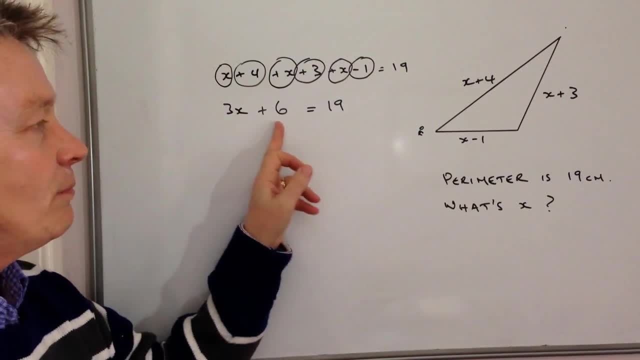 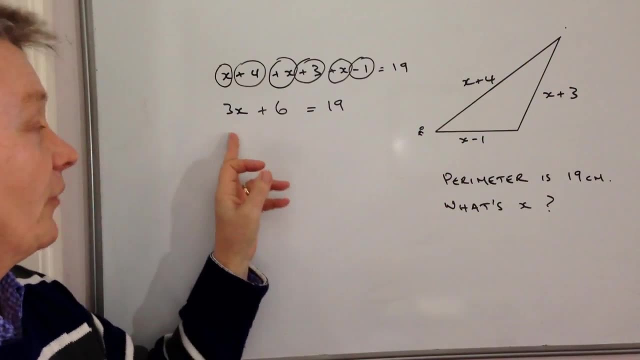 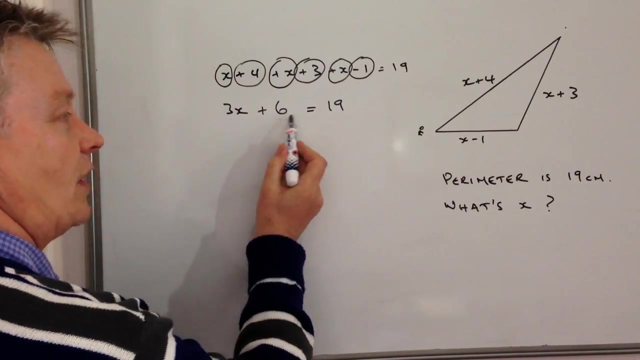 over there. so what we're saying really is that a simplified version of all of this information about this triangle, the perimeter of this triangle, is that that's a simplified way of putting everything okay, and then it's a case really of solving this to find the value of x itself. so 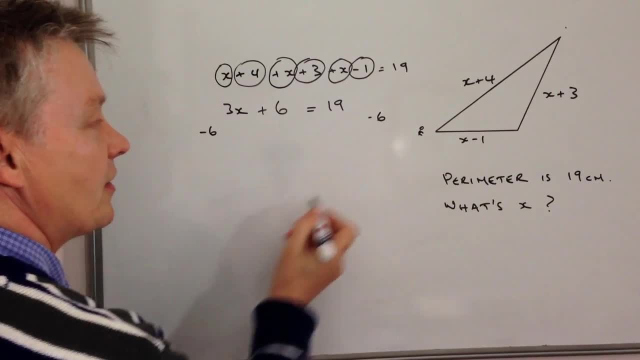 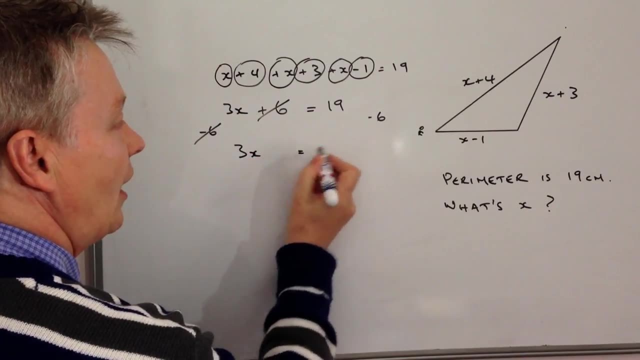 what I'm going to do is I'm going to minus 6 from both sides, because if I do that, it means this will cancel out, and on the left hand side I end up with 3x and on the right hand side I end up with 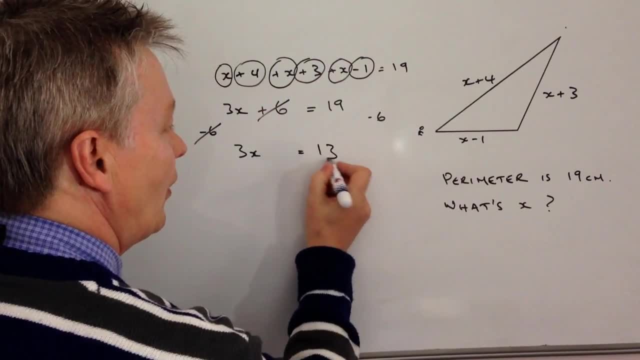 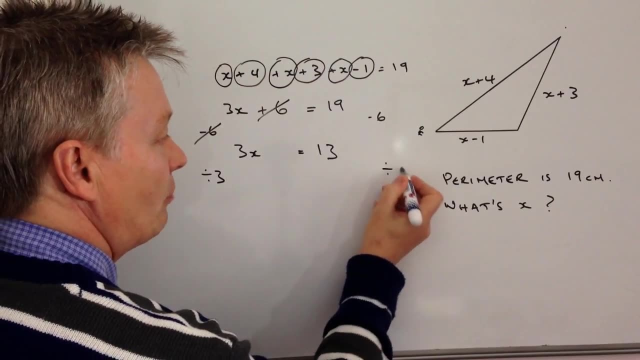 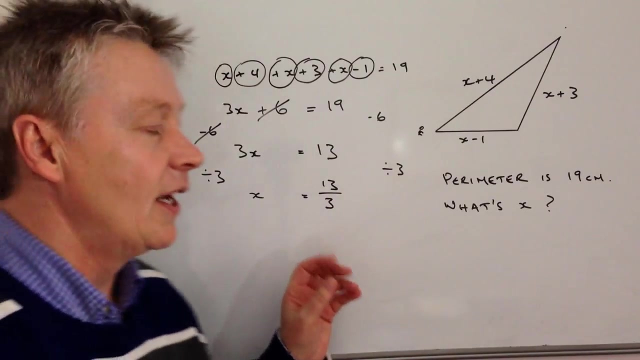 19 minus 6, which is 13. so 3 lots of x equals 13. and then if I divide through by 3 both sides, I end up with x on this side, and this is 13 divided by 3. Okay, well, you can either leave it at that, if you wanted to. 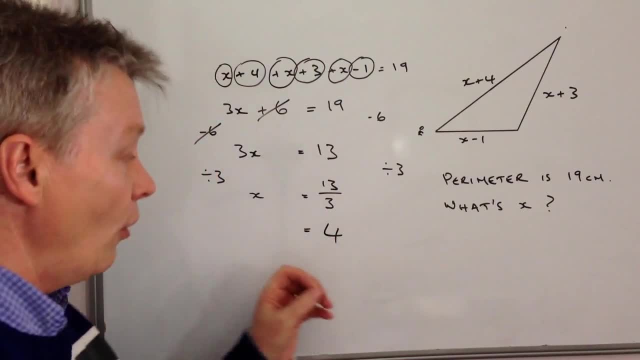 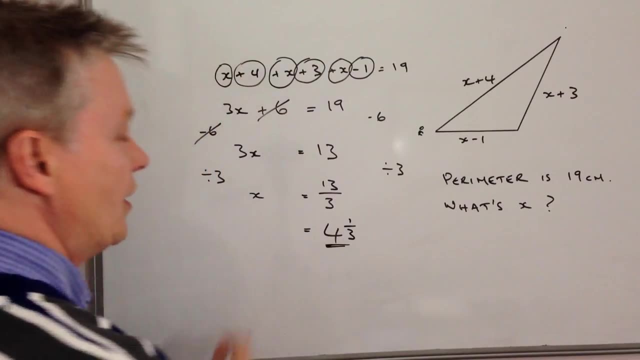 or you could write it as a mixed number, which is 4 holes, because 4 times 3 is 12, and then 1 third left over. So x is either 13 over 3, or 4 and 1 third.